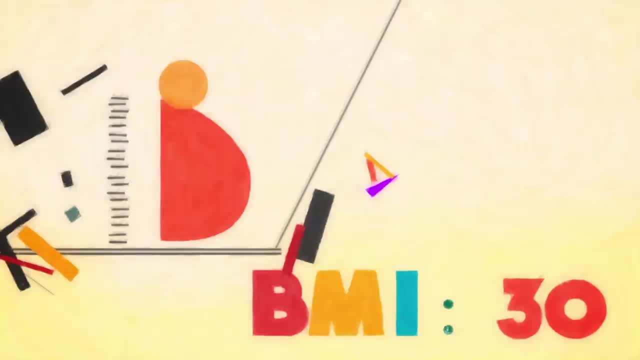 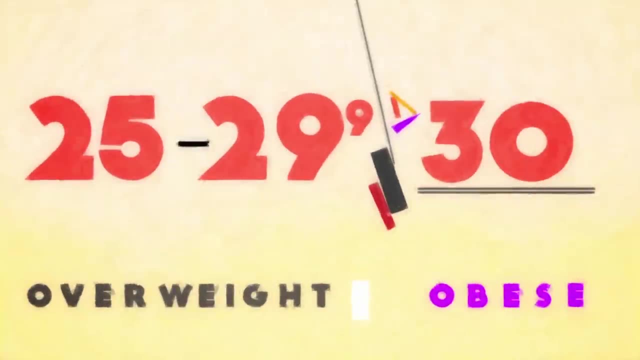 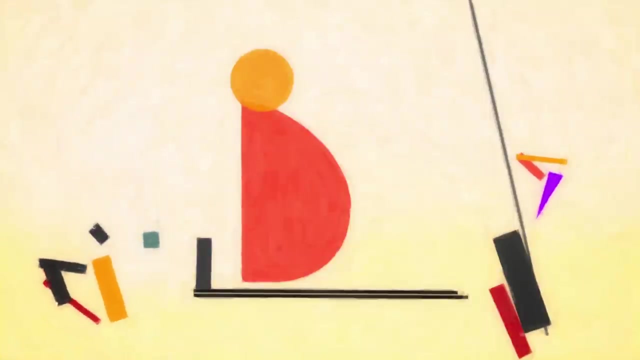 Obesity is a condition of excess body fat that occurs when a person's BMI is above 30, just over the overweight range of 25 to 29.9.. While BMI can be a helpful estimate of healthy weight, actual body fat percentage can only really be determined. 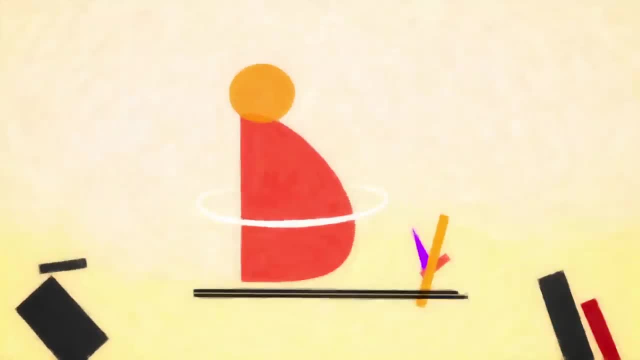 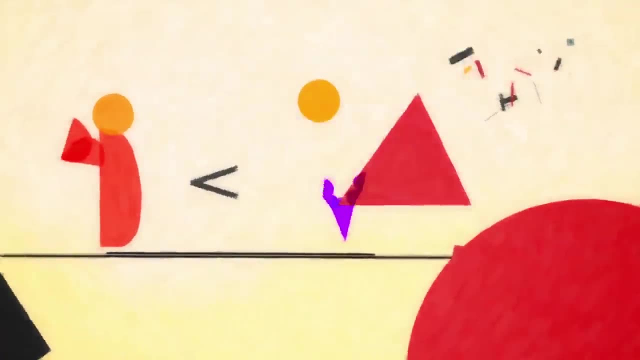 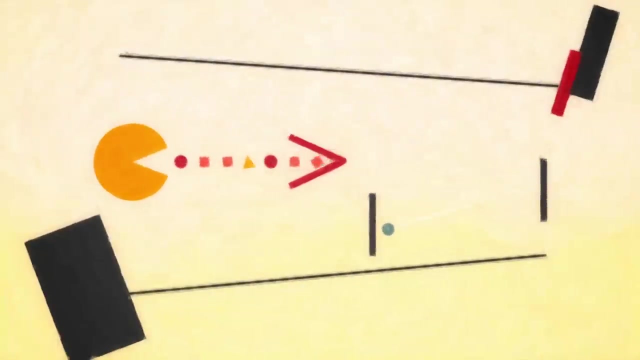 by also considering information like waist circumference and muscle mass. Athletes, for instance, have a naturally higher BMI. So how does a person become obese? At its most basic, obesity is caused by energy imbalance: If the energy input from calories is greater than the energy output from physical activity. 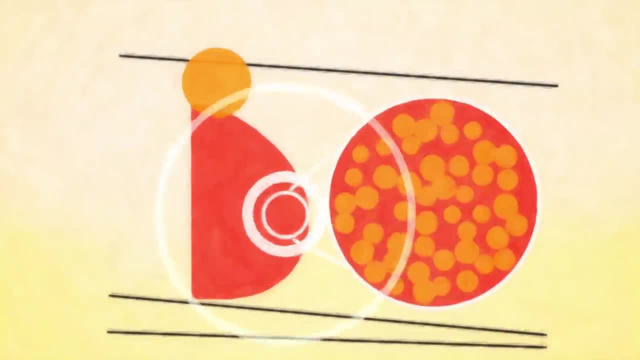 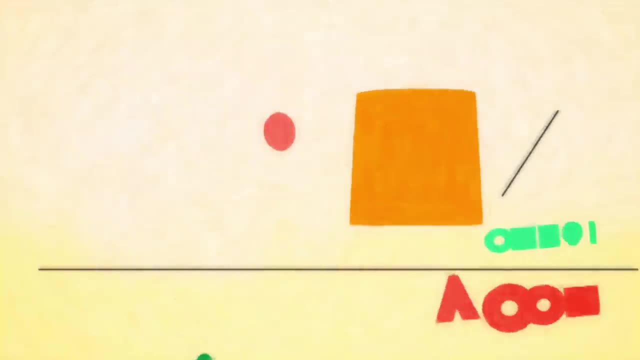 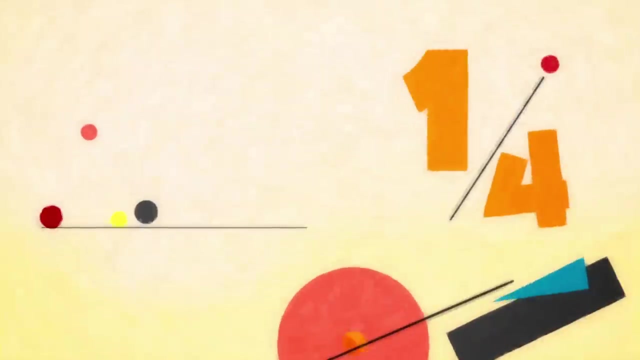 the body stores the extra calories as fat. In most cases, this imbalance comes from a combination of circumstances and choices. Adults should be getting at least 2.5 hours of exercise each week and children a whole hour per day, But globally, 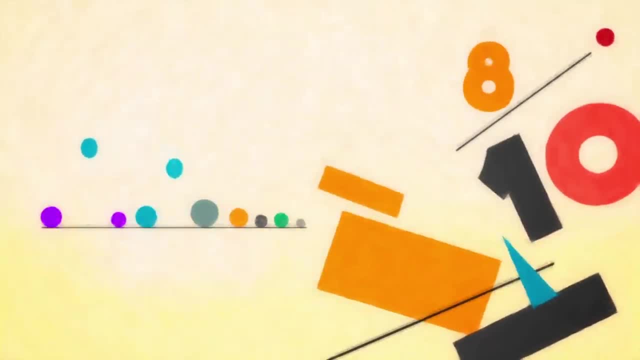 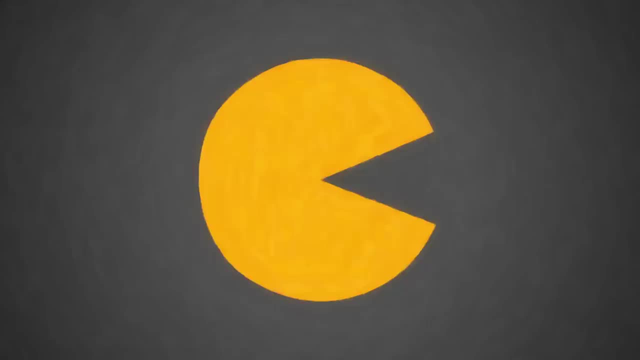 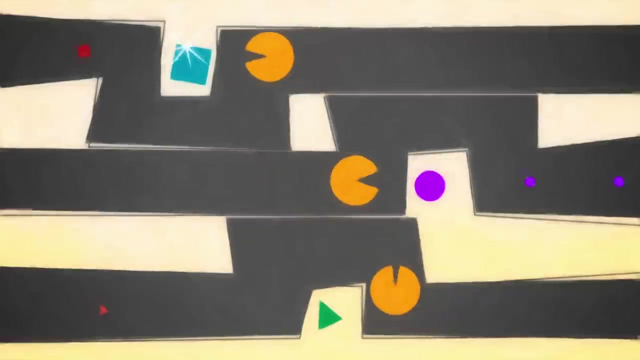 1 in 4 adults and 8 out of 10 adolescents aren't active enough. Calorie-dense processed foods and growing portion sizes, coupled with pervasive marketing, lead to passive overeating And scarce resources and a lack of access to healthy, affordable foods. 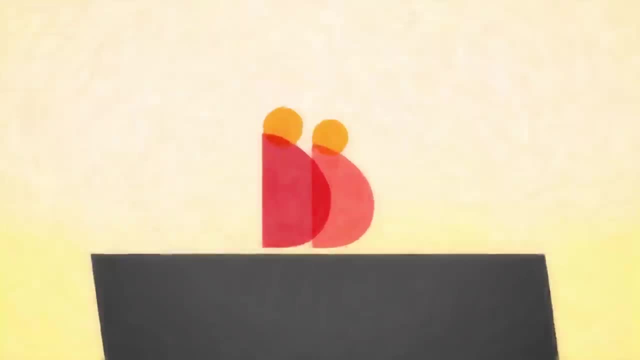 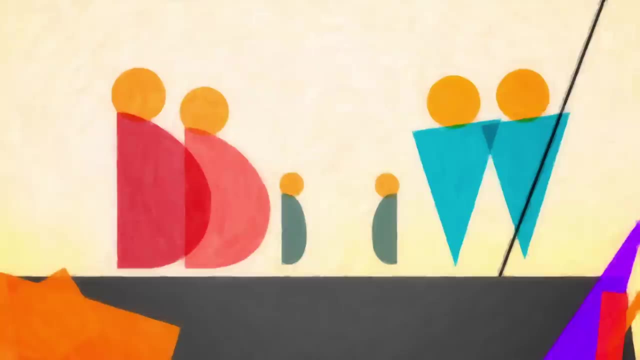 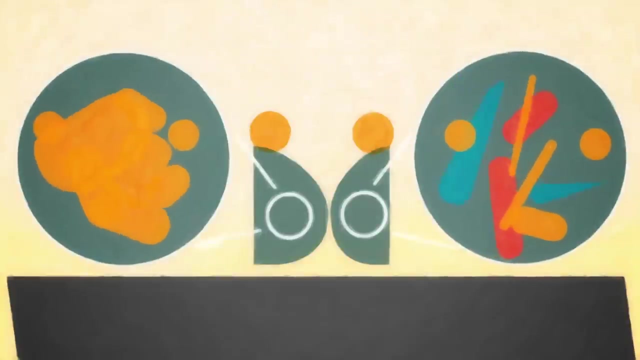 creates an even greater risk in disadvantaged communities. Yet our genetic makeup also plays a part. Studies on families and on separated twins have shown a clear causal hereditary relationship to weight gain. Recent studies have also found a link between obesity and variations in the bacteria species that live in our digestive systems. 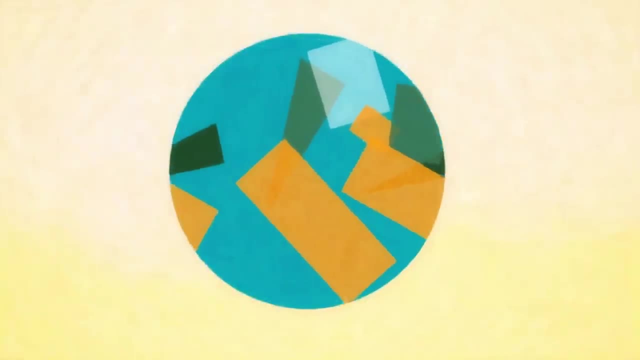 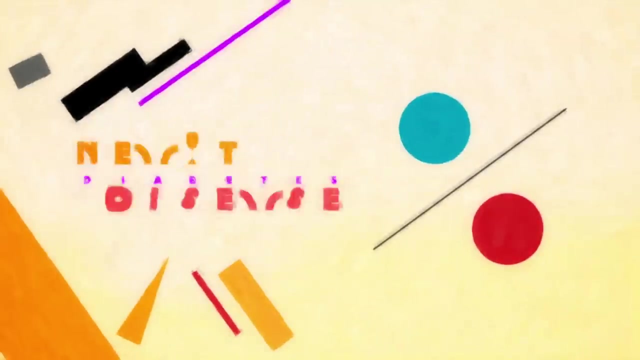 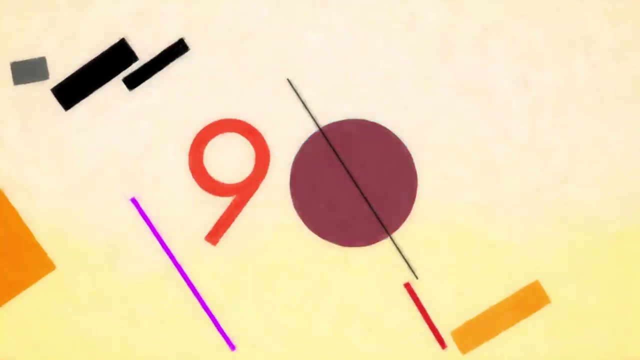 No matter the cause, obesity is an escalating global epidemic. It substantially raises the probability of diseases like diabetes, heart disease, stroke, high blood pressure and cancer. It affects virtually all ages, genders and socioeconomic groups in both developed and developing countries. With a 60% rise in child obesity globally over just two decades, the problem is too significant to ignore. Once a person is obese, the climb to recovery becomes progressively steeper. Hormonal and metabolic changes reduce the body's response to overeating. After losing weight. a formerly overweight person burns less calories doing the same exercises as a person who is naturally the same, Making it much more difficult to shed the excess fat. And as people gain weight, damage to signaling pathways makes it increasingly difficult for the brain to measure food intake. 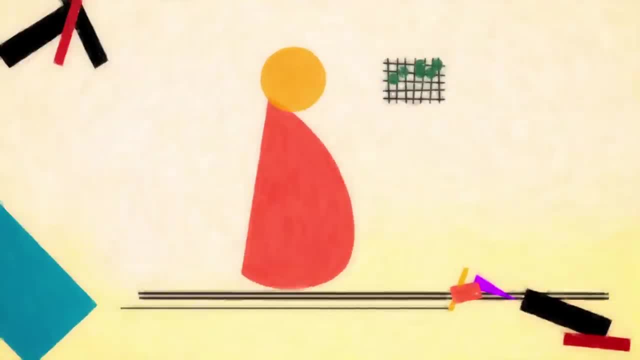 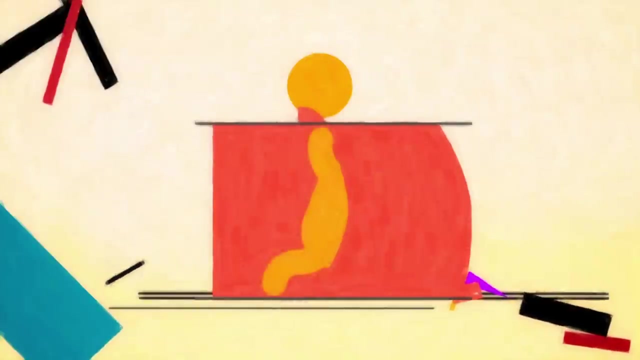 and fat storage. There is, however, some evidence that well-monitored long-term changes in behavior can lead to improvements in obesity-related health issues And weight loss from sustained lifestyle changes or invasive treatments like bariatric surgery can improve insulin resistance and decrease inflammation.